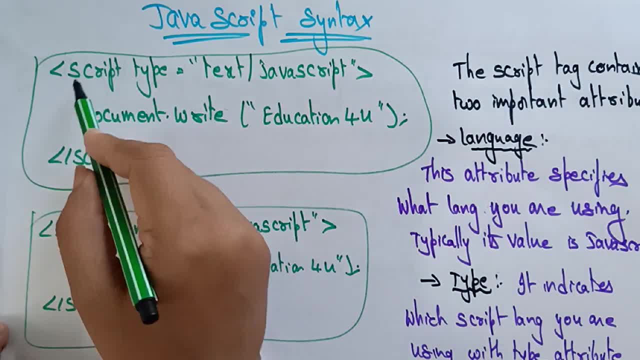 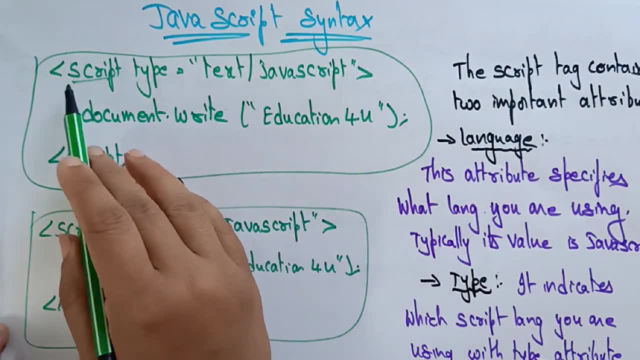 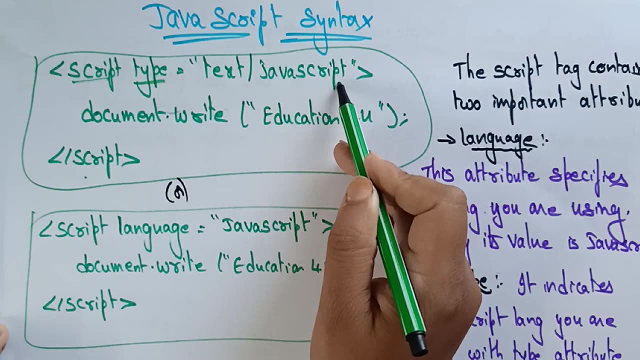 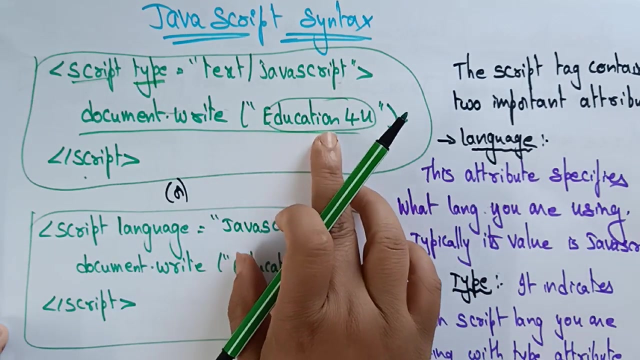 Okay so the JavaScript is with a scripting tags: the scripting script open tag and well as the close tag. Okay so in inside the script you need to write type- Type is equal to text or JavaScript Document dot write. Document dot write is nothing. but whatever the message that you have written inside this document dot write that will be displayed as an output means it's writing the information. 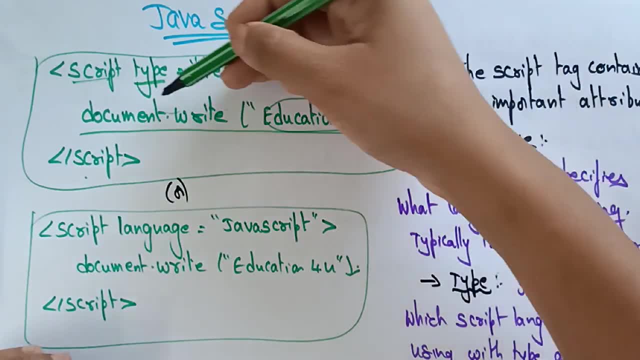 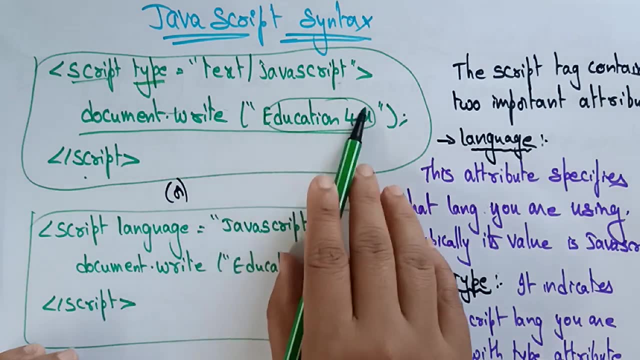 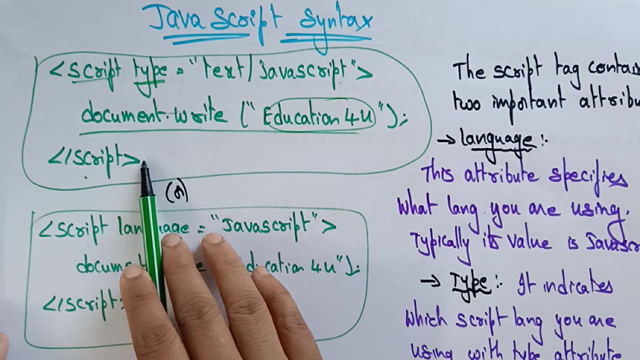 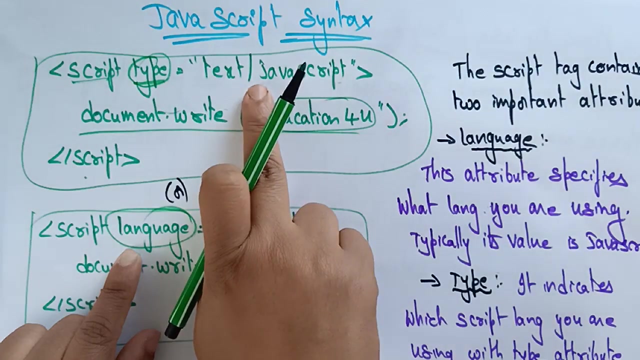 You want to display some information On the screen, that information you have to write inside this document. dot write. So document, dot write. is you have written education for you. Okay, that will be print out. output is print as just simply education for you and script close. or also, instead of type, you can write the language also. Instead of type, you can write script language also. So, while you're written language here, you simply write JavaScript, Don't write text. 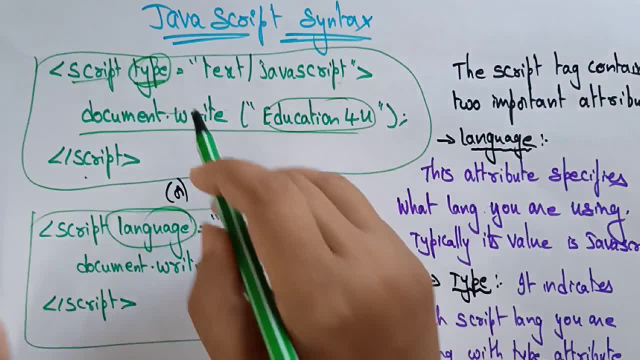 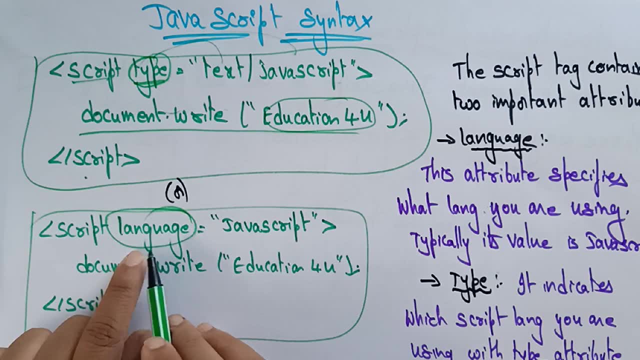 So this, so it's better to take type. If you take type, the type may be a text or type may be a JavaScript. Suppose: if you're written, language means compulsory, you need to write the JavaScript, Don't write the text here. So here the attribute script language is equal to JavaScript and this, everything is the same document. dot write education for you. script close. So the JavaScript was also always having the starting script and ending script tag. 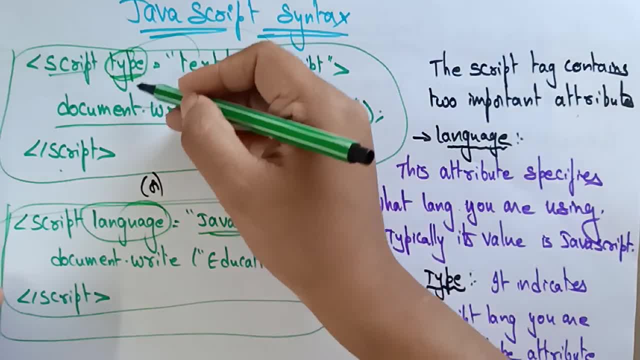 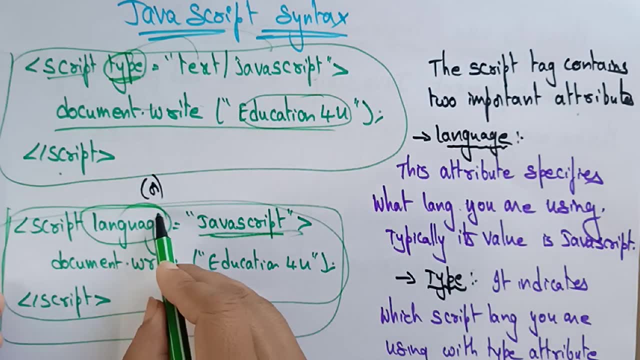 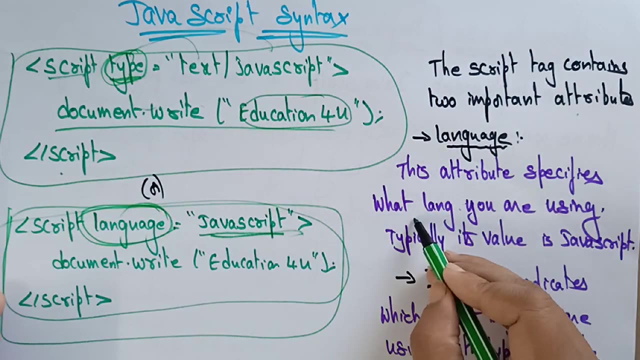 This script tag contains two important attributes. So just now I said it's having two important attributes. So what are those two important attributes? That is, a language and the type. So one attribute is a language and another attribute is the type language. This attribute specifies what language you are using. Okay, so what I what this is saying, what the information it is giving. So script language is equal to JavaScript. It implies that 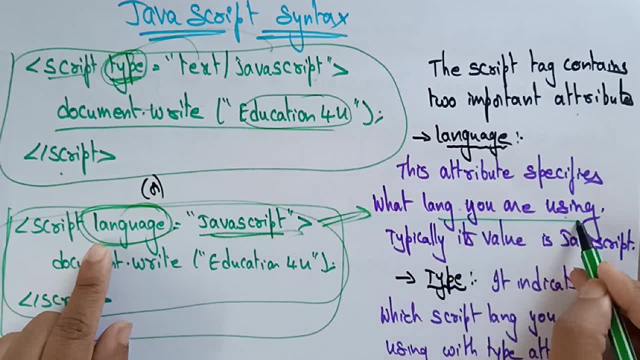 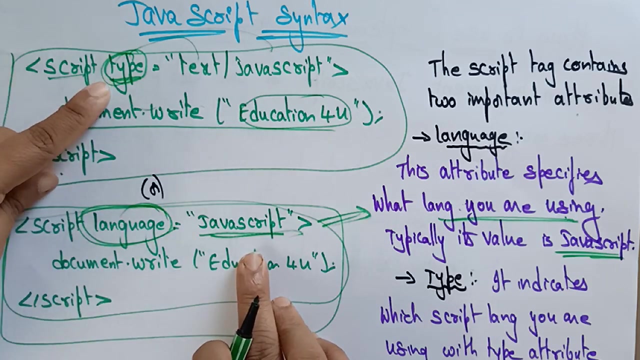 So what language I'm using? I'm using the JavaScript. If you are using any other scripting language, just mention that language, But here, default, I'm using script. language is equal to JavaScript, So typically its value is JavaScript. only Language is equal to JavaScript. Okay, then, if you write the attribute as type instead of language, if you write the attribute as a type type,